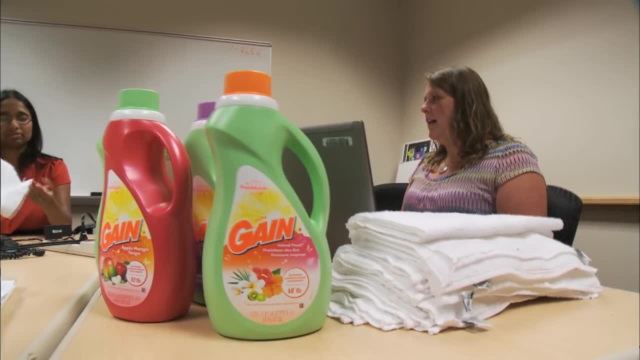 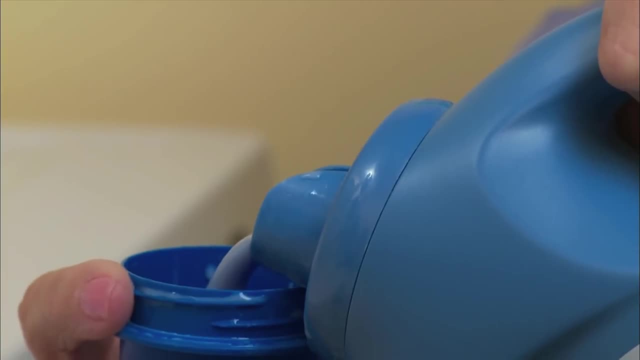 They also talked about how, when they go into their laundry room, they love the smell of that fresh scent and pulling it out of their dryer and being able to smell it. As we're going and investing in the project, we want to make sure that whatever we do is. 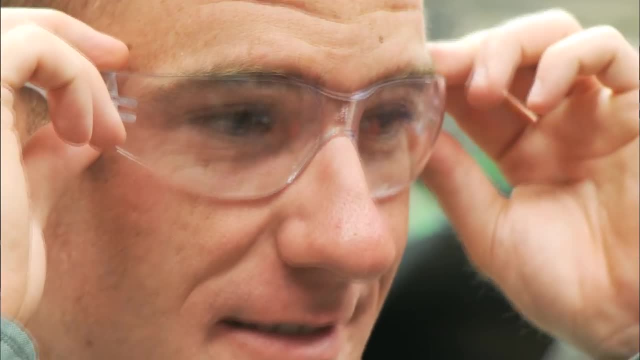 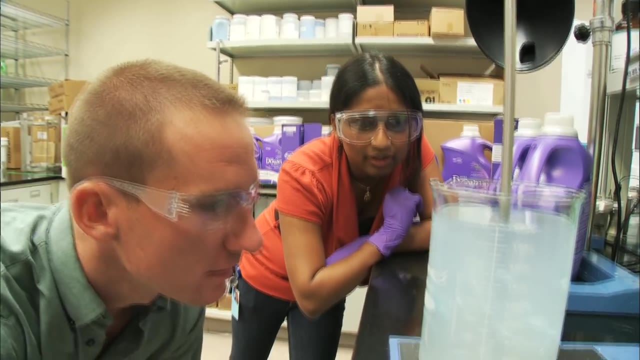 what the consumer wants. Chemical engineers are instrumental early on in the process, Especially during the research and development phase. You've made it in a beaker and that's really cool, But we know we need to make it into many, many, many bottles. 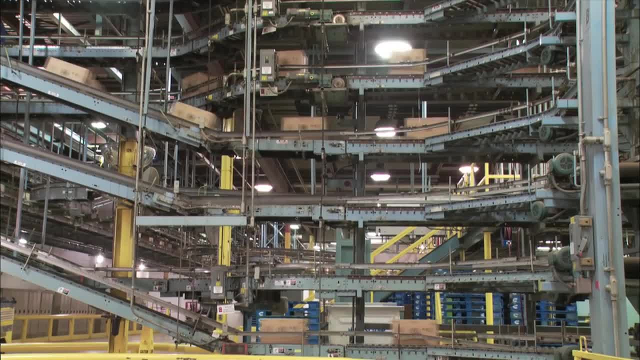 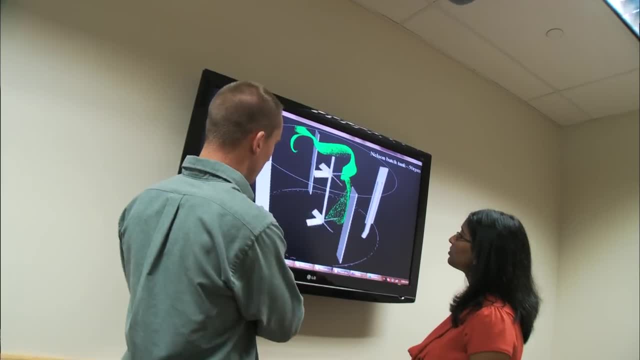 Thousands of bottles that we can get to the consumers every day. So how do we scale that up? With our computer modeling tools? what we've done is we're simulating the injection of this material into our product, So we're showing that it's really well mixed right now. 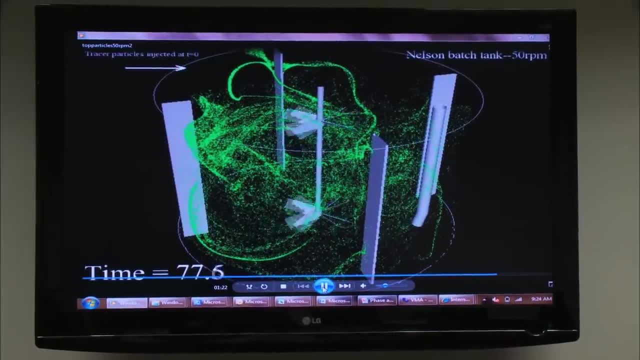 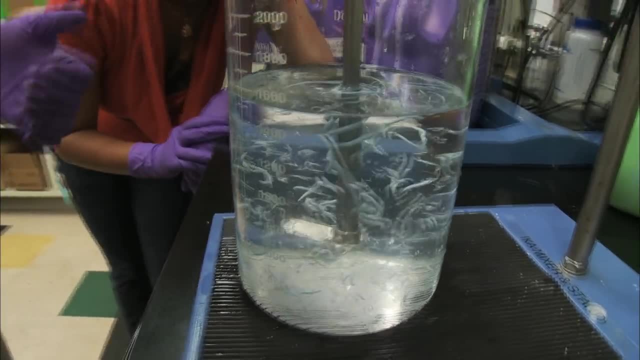 I think that's going to be really important for us making our design requirements, that we know we can get this Now. we can see the rotational movement of the agitator drawing the fluid down, just like the model predicts. Yeah, I can see it going around getting mixed. 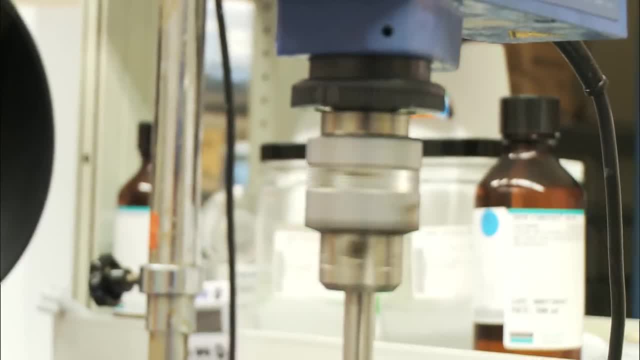 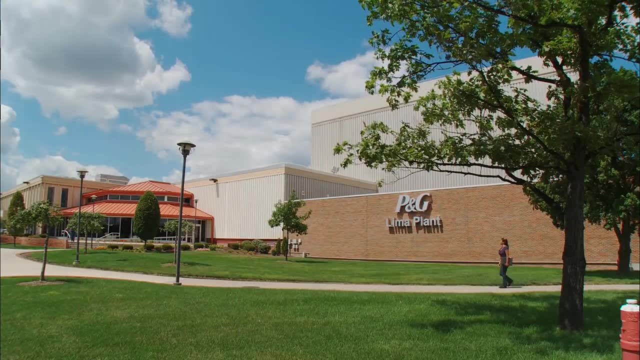 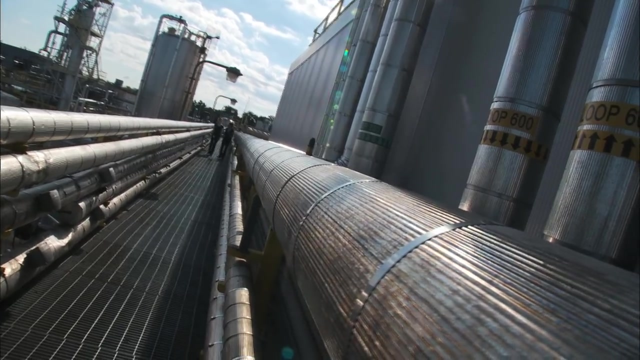 Right And we can see that the strands are breaking up and being drawn down into the fluid And after a few minutes we should see the material dissolve. When Anita's not meeting with her R&D colleagues in Cincinnati, she's usually working at one of Procter & Gamble's manufacturing sites. 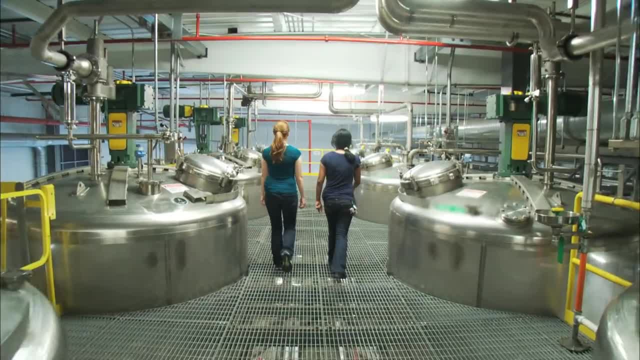 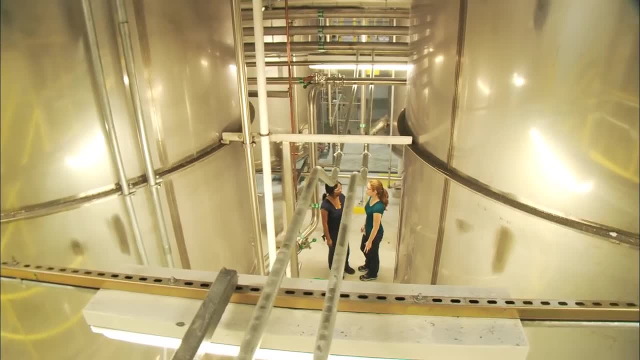 Anita is brainstorming with Lauren, another chemical engineer, planning the scale up of a new product. This tank right here is free. Probably have to do some changes inside. I mean, what kind of material properties does this have? So we're thinking this is going to be a kind of thick material. 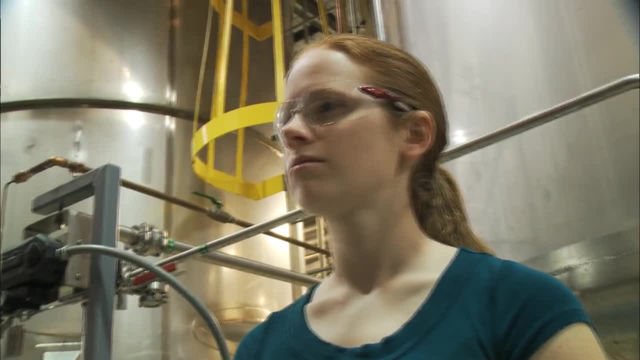 Okay, And we're going to plan to inject it back into our formulas. We want to make sure it's homogenous, Okay, so we're looking at an agitator, maybe a top-mounted or side-mounted one, So it looks like a top-mounted. 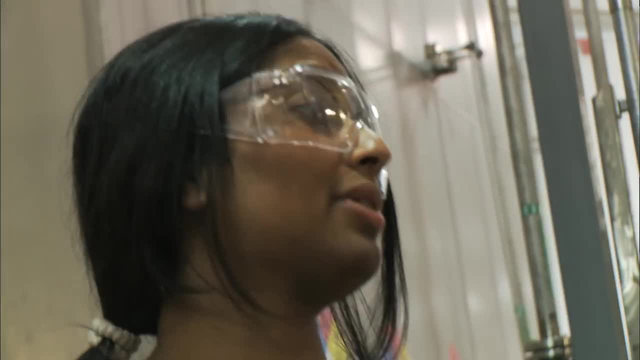 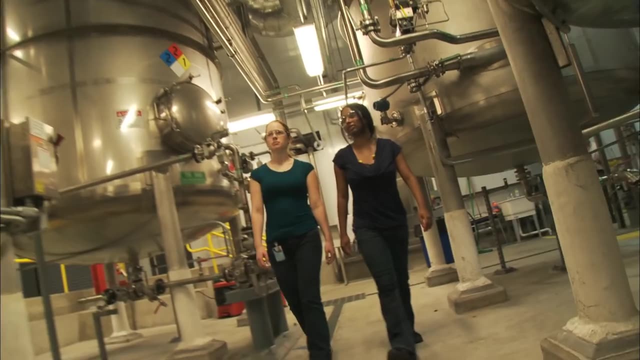 Okay, A top-mounted is what we're going to want. Okay, That's how we're avoiding phase separation. right now, I pick chemical engineering because it's the most versatile. I can work in product supply. I can work in environment. I can work in the energy sector. 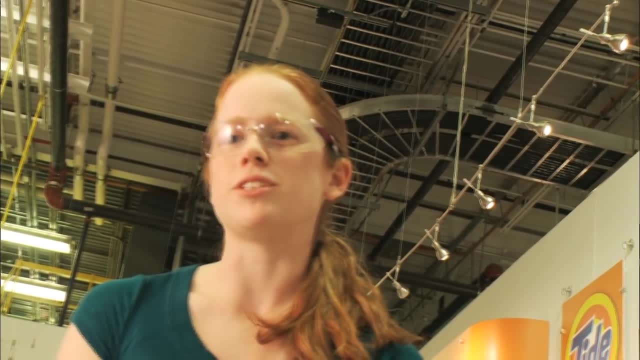 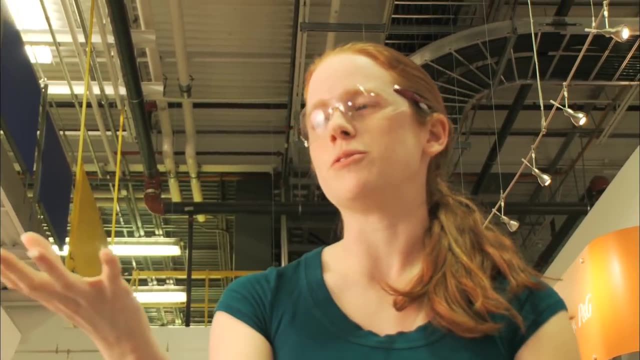 I can work in chemical production. I have so many options. You work all day and you produce these things, but then you go to the store and you see it on the shelf and you're like, oh well, see, I made that. 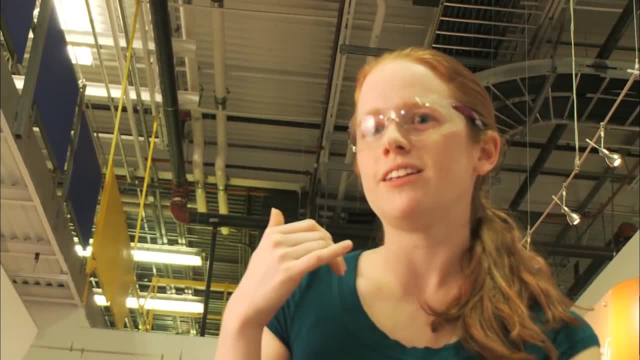 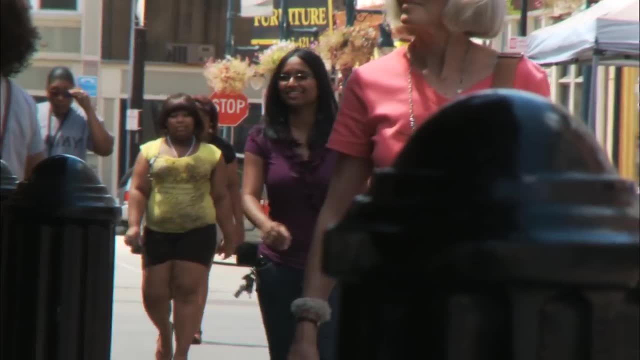 And my mom will call me up and she'll be like: did you make this new thing Awesome? And I'm like, yeah, I did During the day. I'm a chemical engineer, but once I go home I like to do a lot of other. 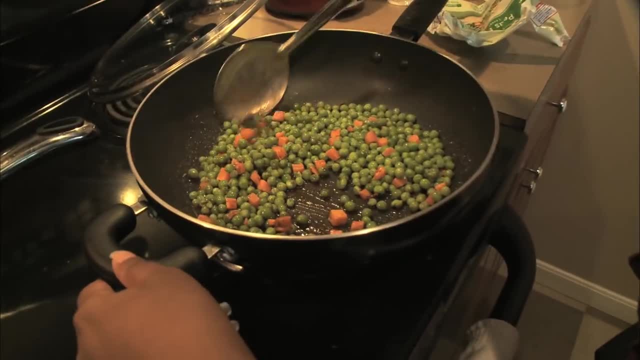 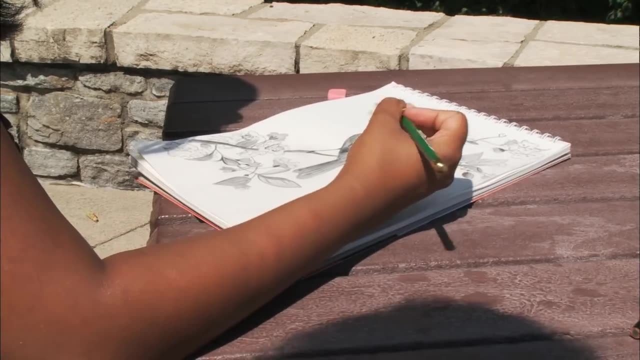 things too. I've learned how to cook and I like trying different recipes out and sharing them with my friends. I like to do different types of art: I paint and I do draw. I think one of the most exciting things about my work is it's not just one project. 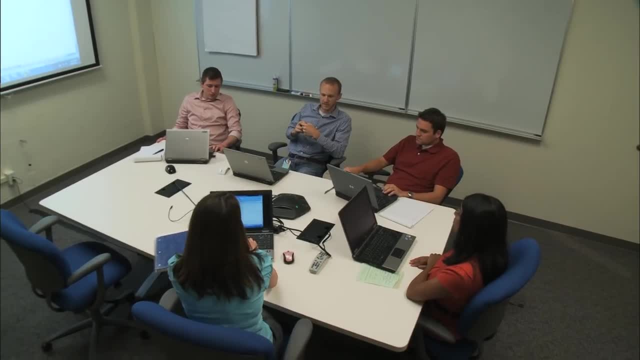 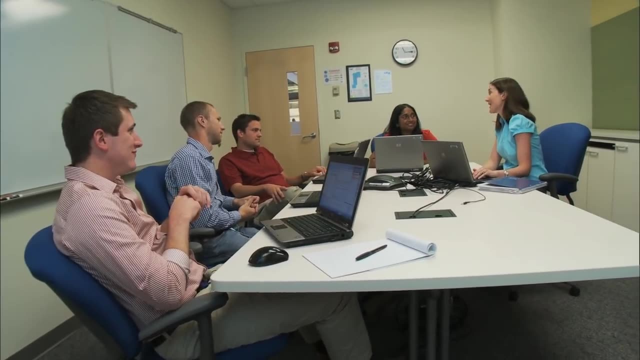 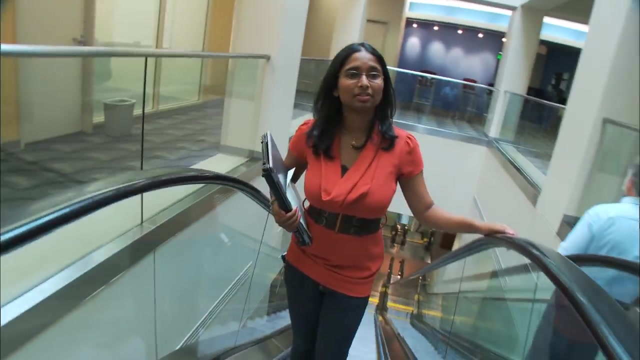 And they might be in different phases. So after several months of options analysis, we have gotten alignment from our GM on a base plan for this project. As chemical engineers design their projects, they take into account consumer preferences, implementation costs and especially plant safety. 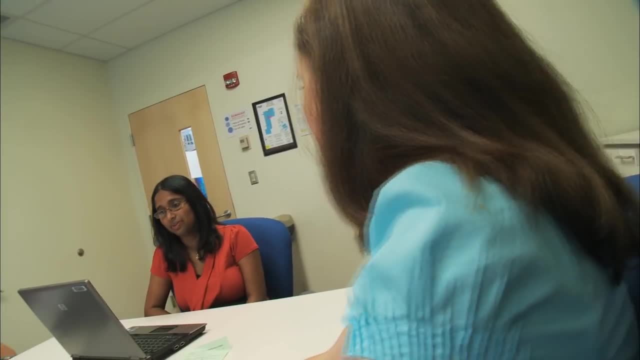 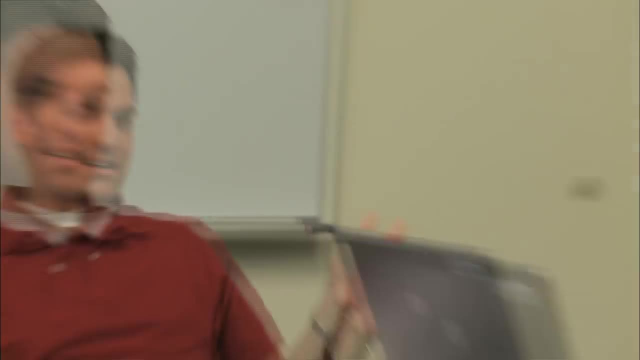 We're working on a noise study. We measured what the sound was actually because, using the site's official destination, We had a system that was supposed to be a possible meter, because we did want to get that recorded. We had it custom made for sound proofing. 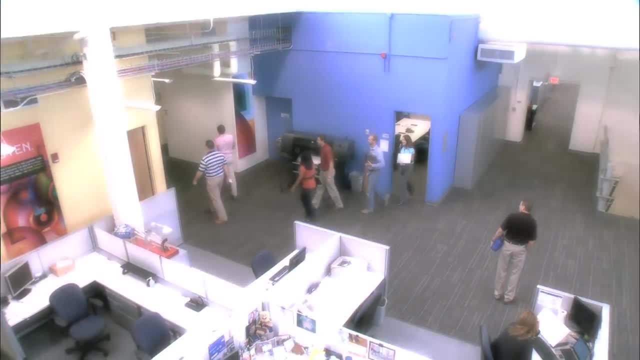 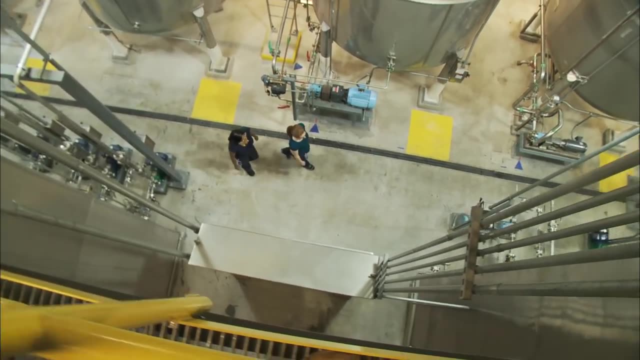 We need noise cancellation. I would research that Chemical engineers also make sure their designs are environmentally sustainable. We're thinking that the batch cycle time is going to take about 75 minutes after unload. Okay, so we want to try to get that reduced as much as possible, if they can. 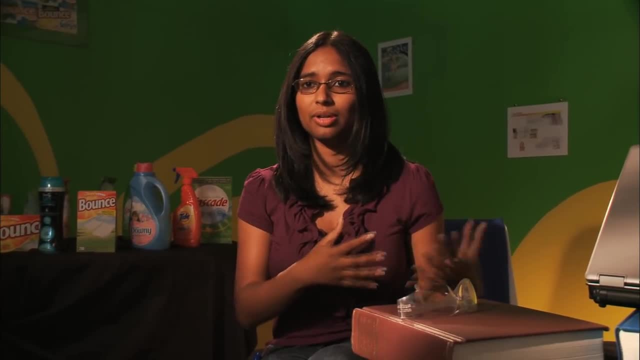 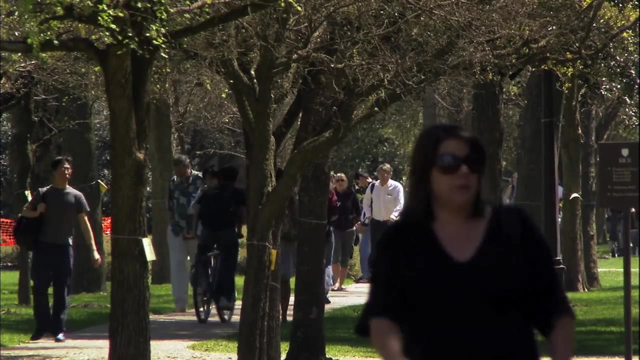 Everything in life is about chemistry and we need to understand how to control it and make it work- And make it work in a clean, green and efficient way. Right Sustainability is a huge thing now. Chemical engineers typically have a bachelor's degree in chemical engineering. 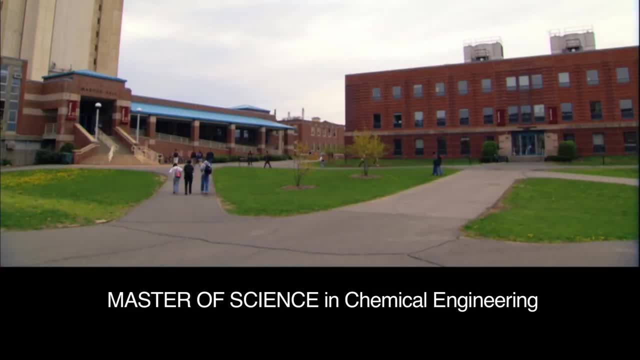 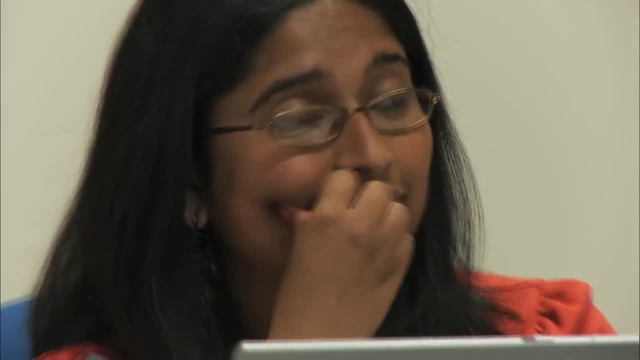 And some go on to receive a master's degree in chemical engineering. But being an engineer isn't just about math and science, you know. You do want to have a good basis in other things like history and English and being able to communicate well.